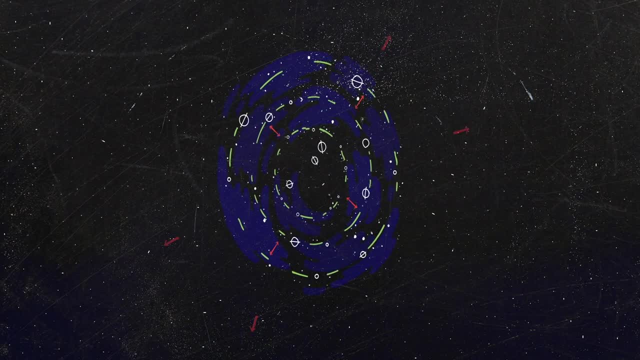 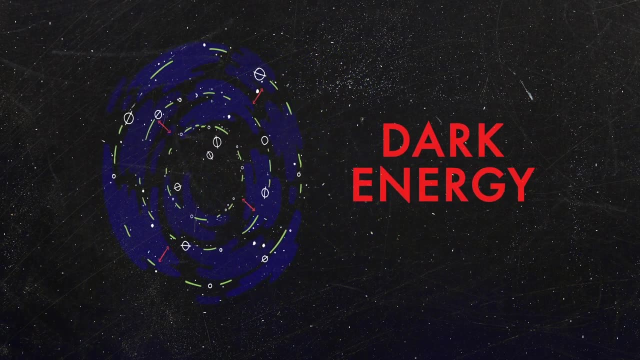 The galaxy itself is not getting bigger. The Earth is not getting bigger. It's the empty space in between, And we think that's the end of the universe. That's due to something we call dark energy. We don't really know what dark energy is. 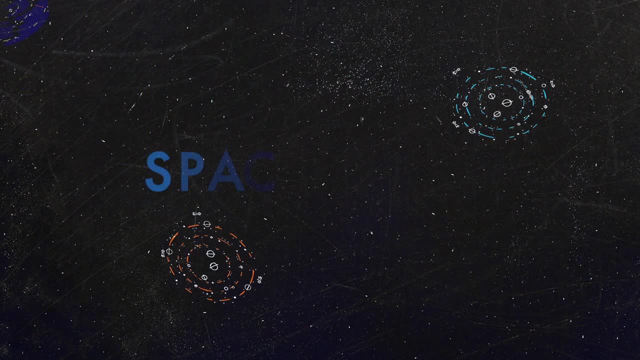 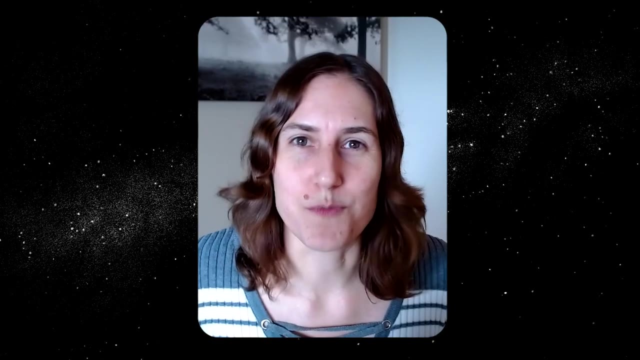 but our best guess is that it's a cosmological constant, which means it's a basic property of space-time, where there's just this kind of inherent stretchiness in space. And so when you have more space, you have more stretching and it's making the universe expand faster. 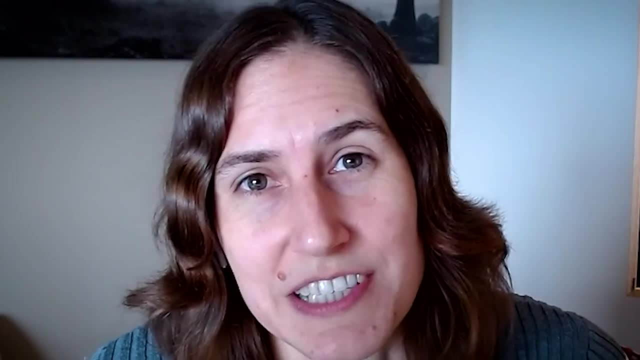 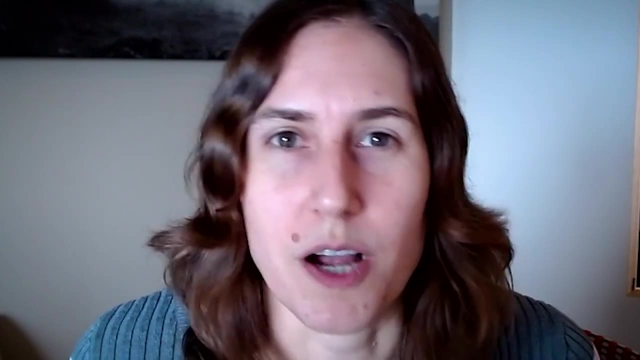 and faster. But there are some other possibilities for what dark energy is, and some of them are a little bit scarier. There's one called phantom dark energy where, instead of just being a sort of property of space that's constant all the time, dark energy is something dynamical, something that changes. 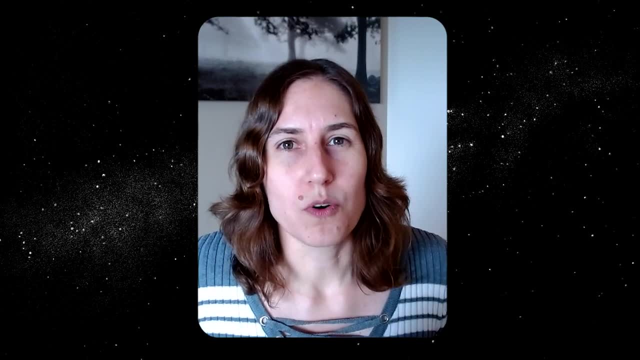 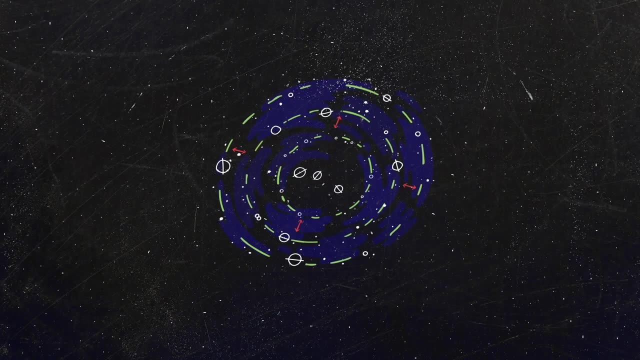 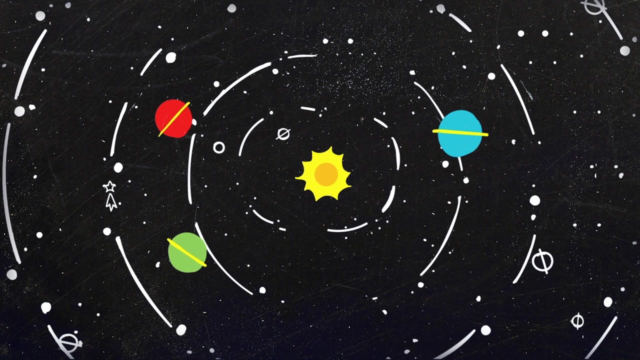 over time in a way that would make it so that there's more dark energy over time, that space is not only expanding in between everything, but starts expanding within objects, within galaxies, within solar systems, And if that's true, that leads us to a really scary conclusion. 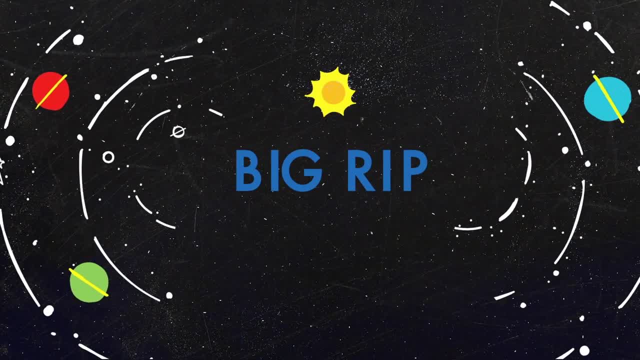 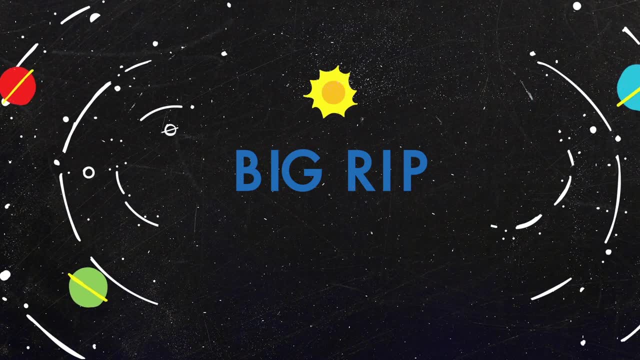 which is that the universe would be heading for what we call a big rip. What that means is that sufficient period of time the universe would start stretching out so much that it would ultimately pull itself apart. And you can calculate, based on what we currently know about the expansion rate. 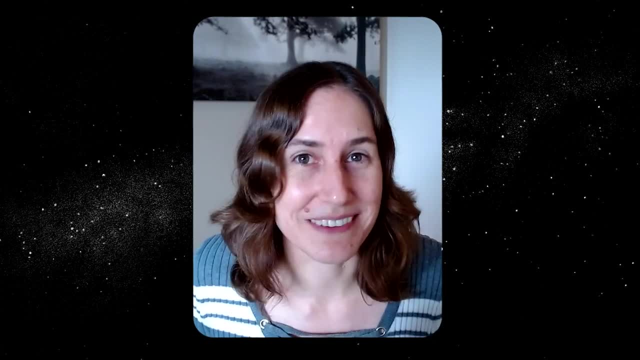 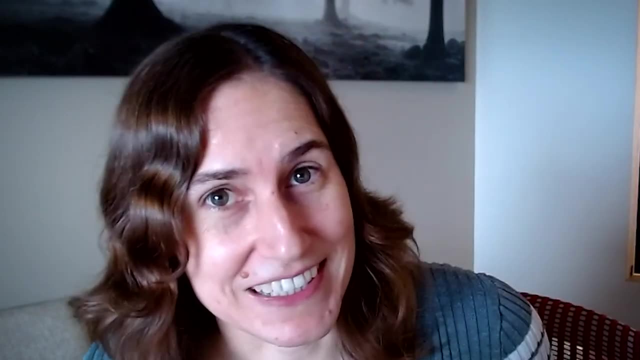 what the earliest. that would be that final big rip end of the universe, And we think it's somewhere around 200 billion years, but probably it's not going to happen. But if it did, then what you would see is you'd first see galaxy clusters coming apart. That would be in sort of the last. 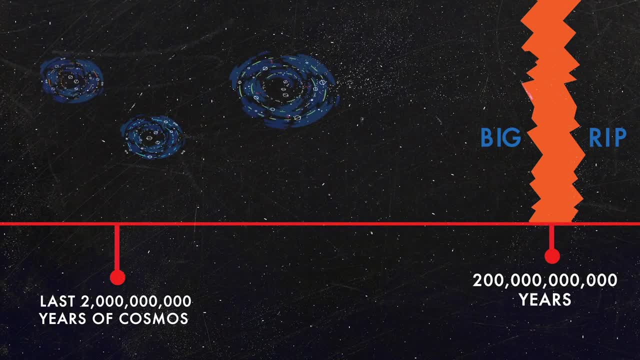 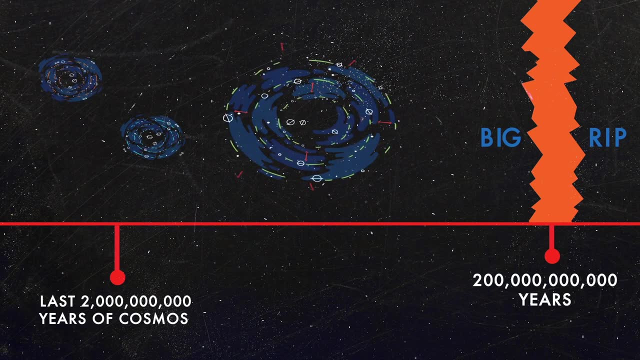 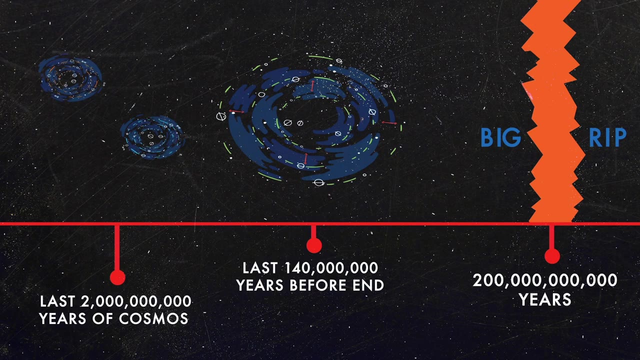 two billion years or so of the cosmos, And then you'd start to destroy galaxies. Galaxies would start to pull apart as the dark energy within them pulls on them from the inside. Stars would start to wander away from galaxies. That would be in about 140 million years before the very. 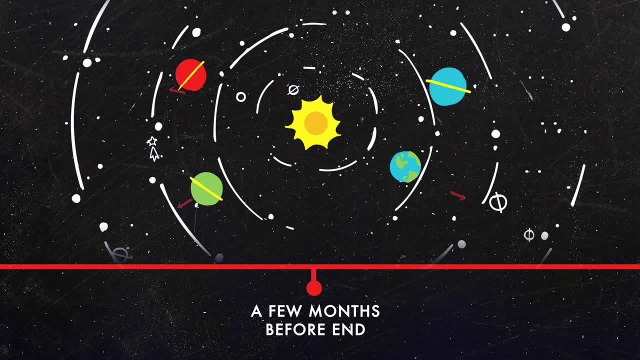 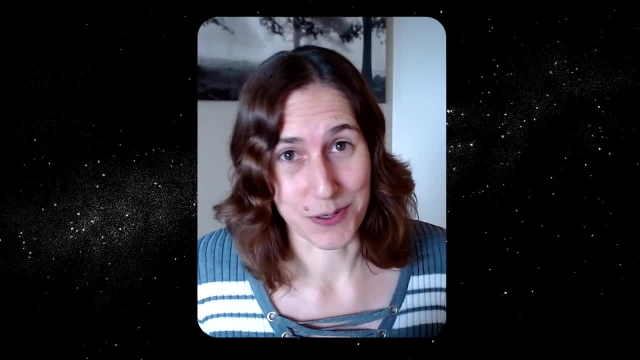 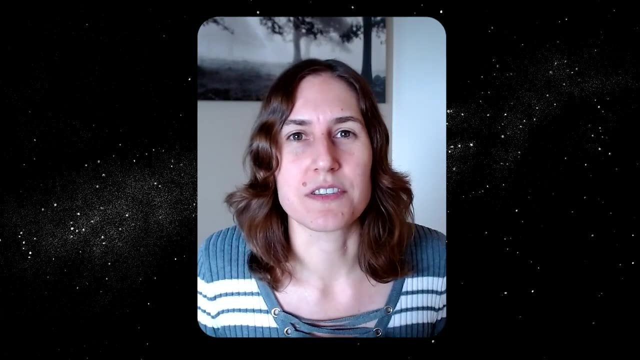 very end, And then, just a few months before the end, you would get the solar system coming apart. Planets would wander off away from the sun, And then it gets really personal at that point, because then Even planets can't hold together anymore. There's so much stretching of space that you would start.